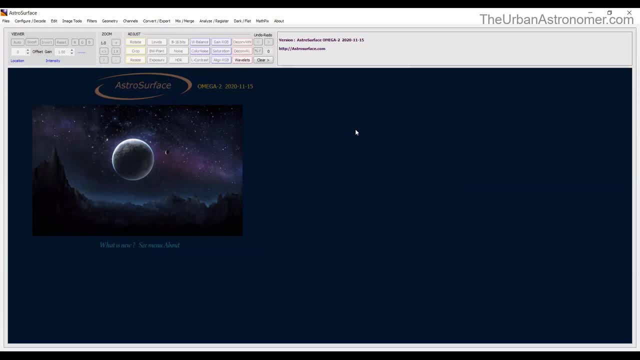 astro surface. so i just want to give a shout out, before we begin, to scott bass. uh, he's the one who actually introduced me to this program, uh, on one of the uh yccd facebook forums, and he actually gave me a list of um steps, uh to just, you know, help me get started on this program. and that was. 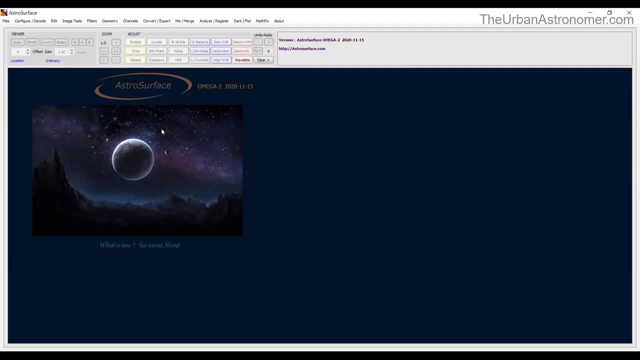 really helpful, because there is a set of steps that you need to do. it may not be completely obvious by just looking at this um, so i don't know, maybe in a future version of the program, maybe over here we can just have an image on what you need to do. 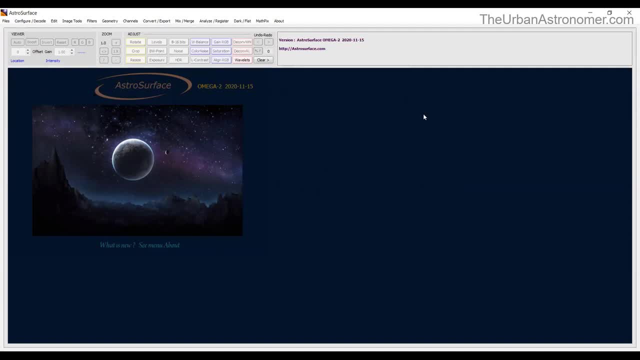 like you know, analyze first, register, analyze stack and so on. but anyways, this, this is a fantastic program. so let's actually dive into, uh, how we can process planetary image, images from planetary videos, uh, basically planetary stacking with astro surface. so, uh, hopefully most of you already know how to do planetary stacking. 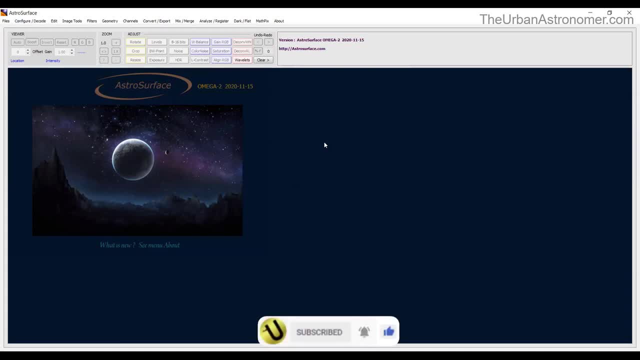 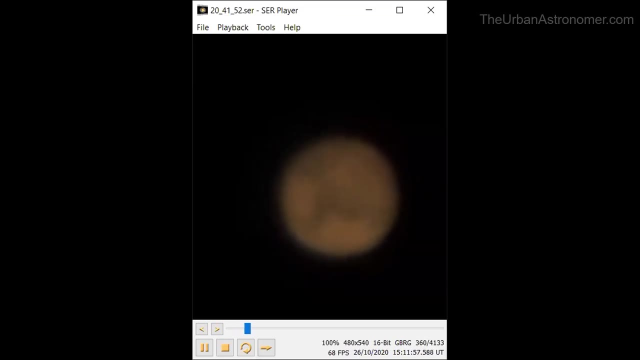 um, if that's not the case, i'm just going to give a? um a brief intro. um, if you're not interested in that again, skip ahead. i i will uh be uh splitting this video into chapters so that it's easy to navigate uh to any part of the tutorial that you wish to see. so the way we actually do uh, 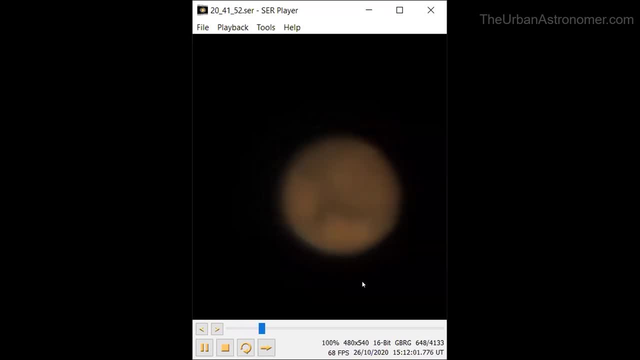 planetary imaging is first we take a footage like this. okay, so to take a video footage of the planets, either you might have an astronomy camera which you will connect to your computer, and then you can use a program like sharp cap, which i have used to capture this particular. 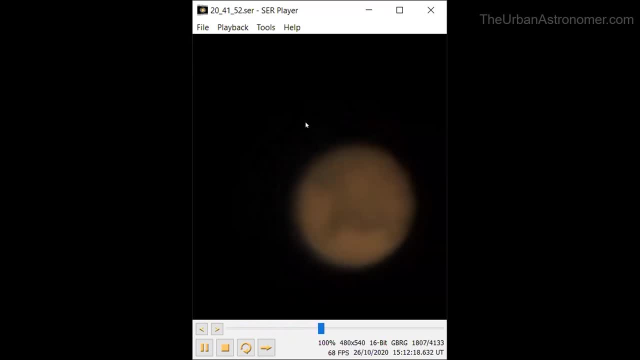 footage. otherwise, you can also use a dslr with a t adapter and a t-ring to connect to the telescope and then use that footage from that, which might usually be stored in an mov file or something. if that is the case, uh, then uh, you will need to, uh actually uh, convert the mov file into an avi file or an acr file. 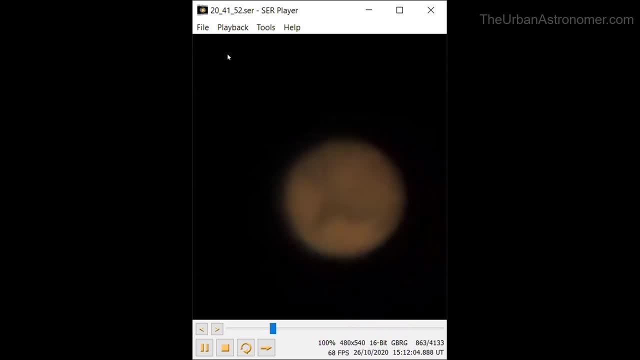 because that is what is needed by most of the processing programs and if you need to do that, you can use a program called pip. this i have already discussed in my earlier planetary videos. i might revise that soon, but any case i will link uh to the latest planetary video, which 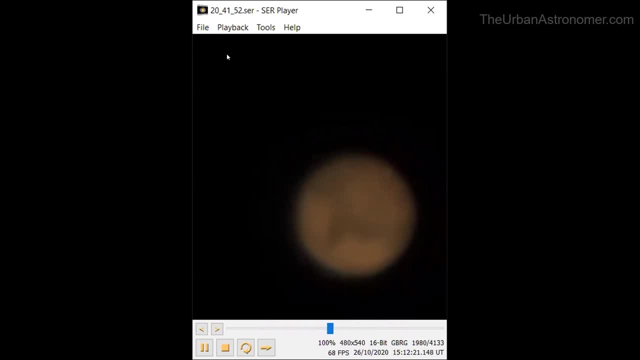 discusses that on this video so you can use the cards to navigate there and check if you want. there's one more option. if you're really just starting out, you have a beginner setup and you don't want to spend additional, you know money on any of like and you don't have a dslr, then 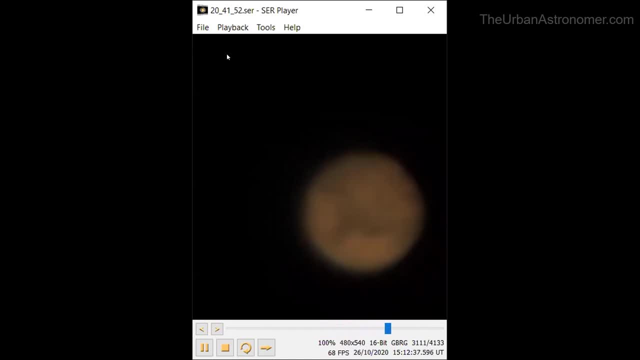 you can actually use a mobile adapter and a mobile phone to actually capture video footage, and this actually depends on the mobile that you have, on how well you can capture the footage and and how good the output is going to be. you can actually get pretty good images, especially for 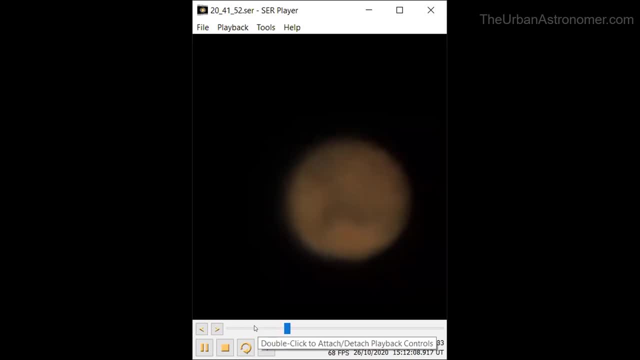 lunar and also for planetary, with just using mobile phones. okay, in that case also, you might want to use a pip to convert that into avis and there are some tips and tricks in pip where you can just enter the- the planet, you know, make the avi file small. so all those i have actually discussed 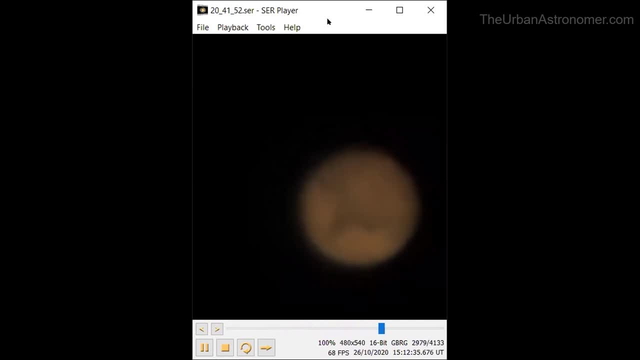 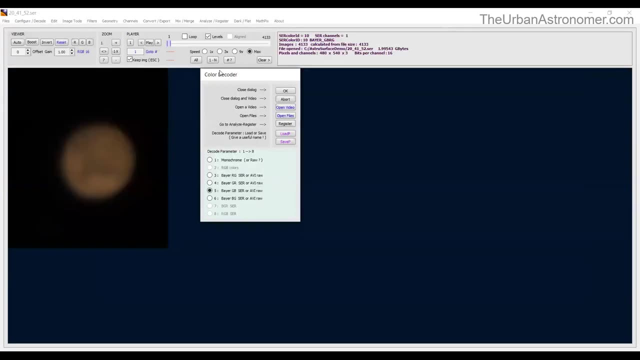 in my other videos. so let's get to uh, processing with astro surface and i will be using this footage. the first step is we will open the footage, okay, and we will get this code decoder dialog and on this dialog, what we need to do is we can actually set the parameters over here, like you do. 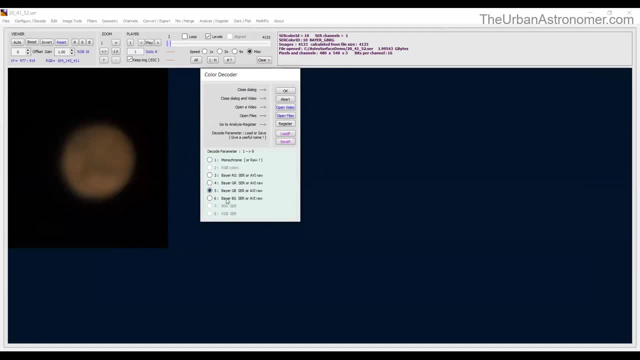 is it a monochrome video? uh, if it is a raw file like acr, or is there a bear pattern, which is basically, when you we have a color image, what bear pattern do we need to use? usually it will just select the default. you can keep that, or then, if you are aware of your bear pattern, you can. 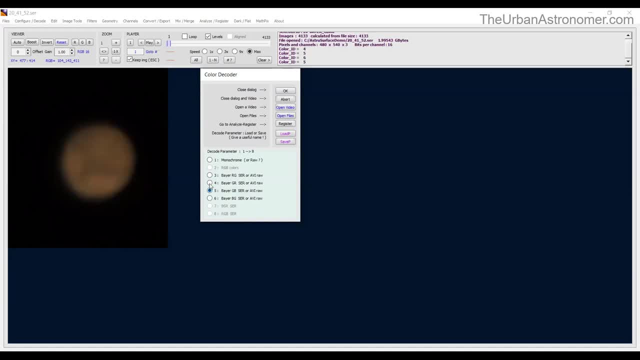 just flip through and make sure that you're getting the correct one as you, as i'm flipping through, you can see that the color over here is changing, so you can make out with that. like, what is the correct bear pattern to use? so in my case it is bear gb, acr or avi raw. i'm going to use that. 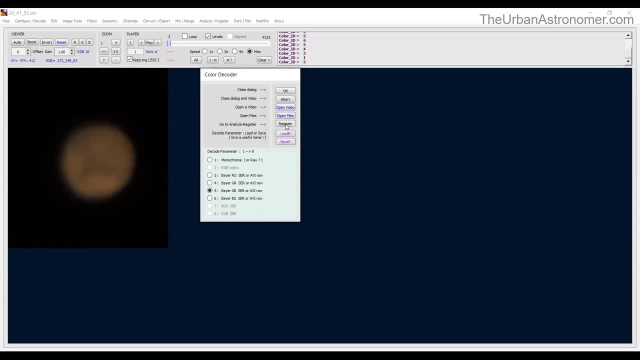 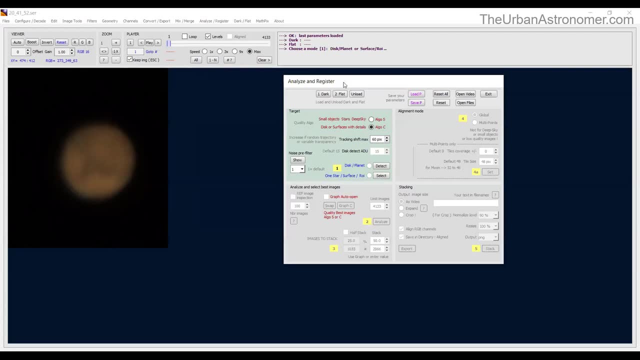 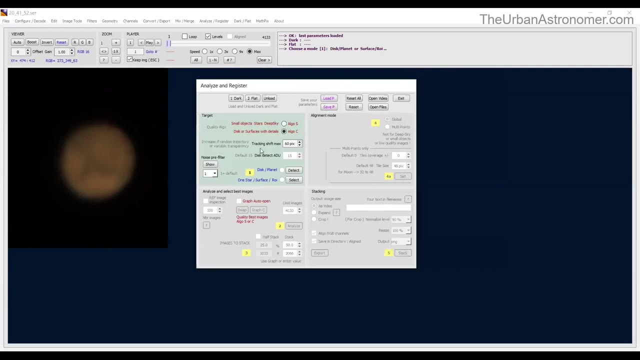 and i'm going to say register, okay. so this is the first step. we have to register the avi or the acr. so when we click on register, we will get this analyze and register dialog. okay, so when we look at this analyze and register dialog, we have two options over here. one: 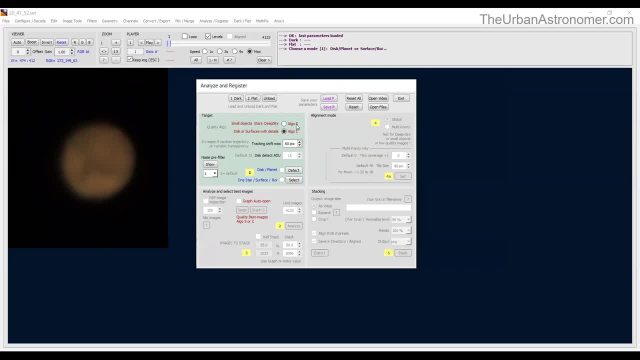 is small objects, stars or deep sky, which is the algorithm s. another one is disk or surface readers with details. so you can see this is a martian disk and usually for planetary you will select disk or surface with details, which is algorithm c, and then we are going to add a space which is called disk planet, and over here there's an option called 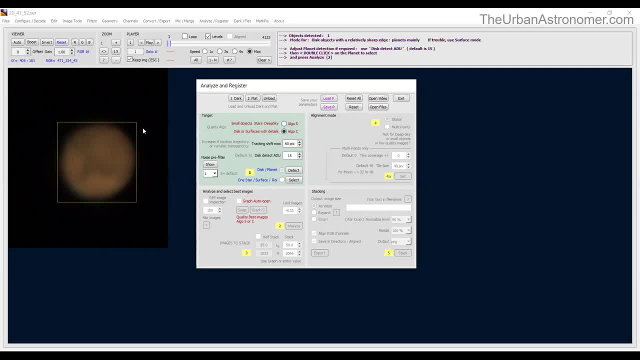 a disk planet. so i'm going to click this and i'm going to click detect over here and that puts a box around the planet and we need to double click that. okay, then that brings about this green box with an additional green box inside that and we can click on analyze. 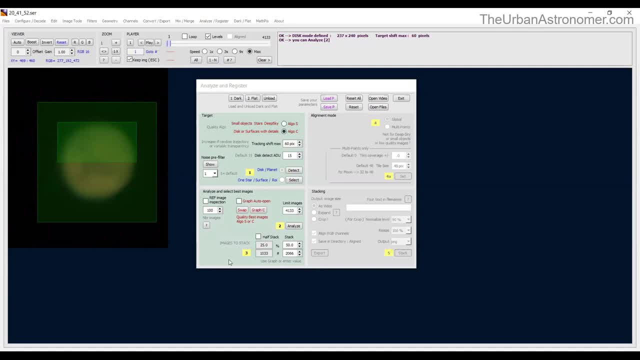 okay, so it? this basically enables the next section. you can see that this section- analyze was not we detect and we double click on the planet. the next section is enabled, which is analyze and select the best images. okay, and, as you see, we can. we have selected algorithm c here and there's a. 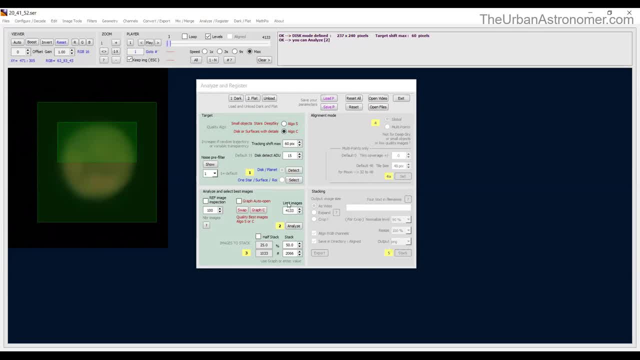 graph c. here we click on analyze and this, this limit image, is basically the total number of frames that i have in the video footage. we click on analyze. so it has analyzed the uh the footage and it has enabled the stacking and the alignment mode uh sections over here you can see there are. 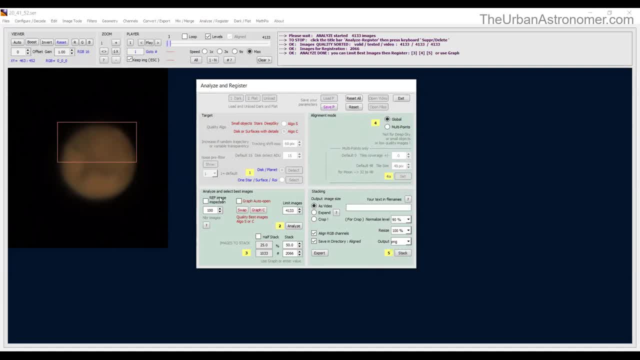 some other images, uh, some other options over here, like reference image inspection and things like that. you can try that if you want. if you need to inspect the reference image, you can do that. uh, there's there. is this graph auto open? so once the analysis is done, it can open the graph. 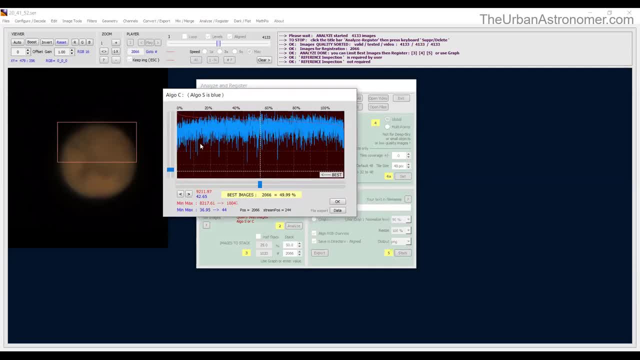 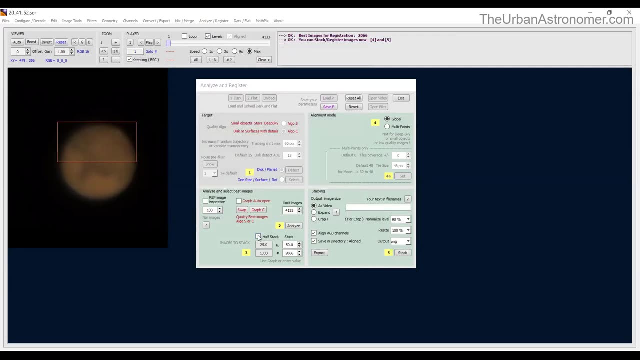 automatically. otherwise you can click on this graph c and it will give you a rough graph that shows what is the quality of the footage that you have. i'm just going to leave this as 50. you can obviously use a slider to move it around and pick what you want. there is also a half stack option. 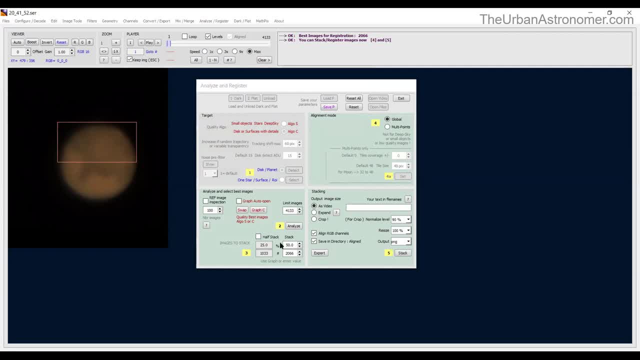 which is, uh, it will stack half of the 50 over here. um, i'm just going to leave that off, i'm just going to use 50 and that means that it will stack around 200 and 2066 frames from my total 4133 frames that it had. that was there in the footage- to stack the. 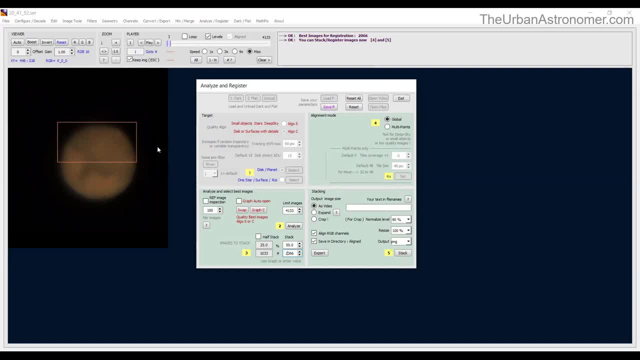 uh, the video, which is basically taking the best frames and then combining all of that into a single image. that is what is stacking right. so to do that, i just need to press stack. there are some options here, so i just chose 90 percent to normalize and then resize as 100 you can. 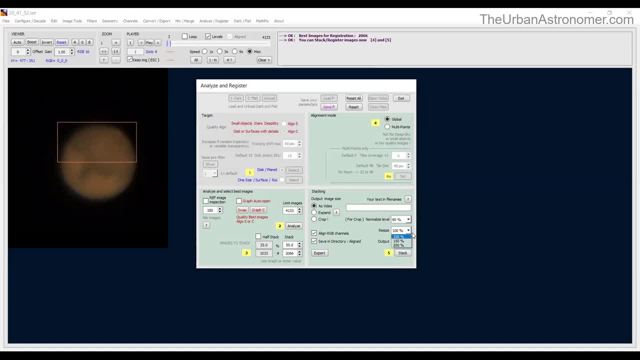 also resize to a. um, if you want a bigger image, you can try resizing into something else like 200, up to 200 percent. uh, what is the output format that you wanted to be? so it can be a png, tiff file, a fit file. uh, i leave it to you, to, you know, choose what you want. i'm just going to leave. 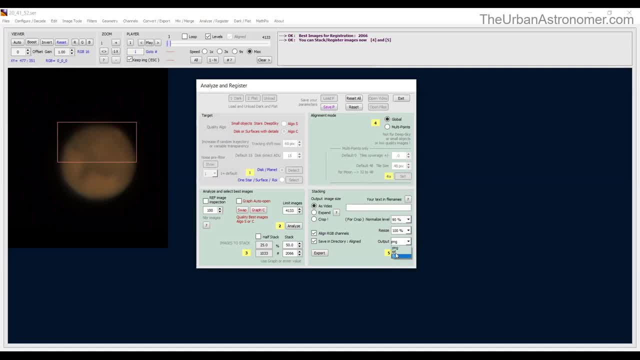 it at png for now, but you can also. you can also use one of the other formats, since you're opening it in uh oster surface itself. uh, there should not be a problem. maybe you can when, while you're saving, you can convert it into the correct format. uh, alignment mode. i'm going to leave as is, which. 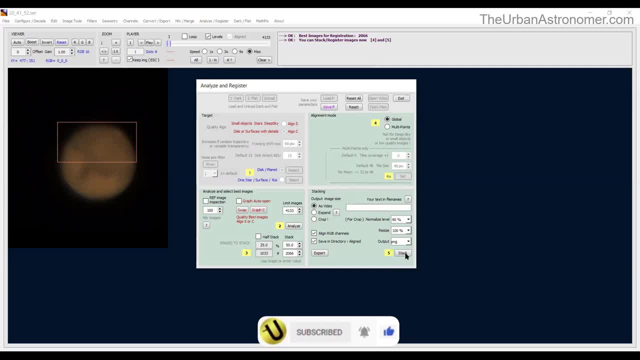 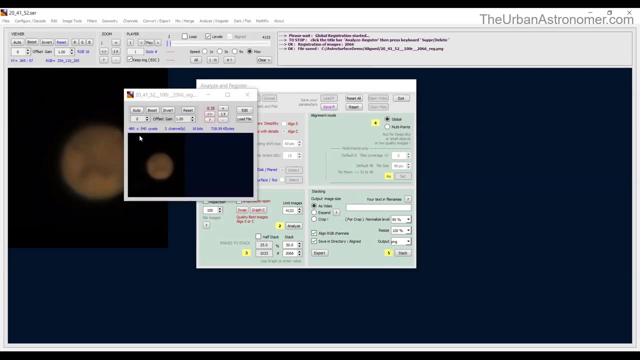 is just using global settings as of now and, uh, you know, it is going to save in a direct recall, aligned in the folder where, uh, the video file is okay, so i'm just going to um stack this. so it has created a stacked image over here, okay, so you can see the stacked version of the image. 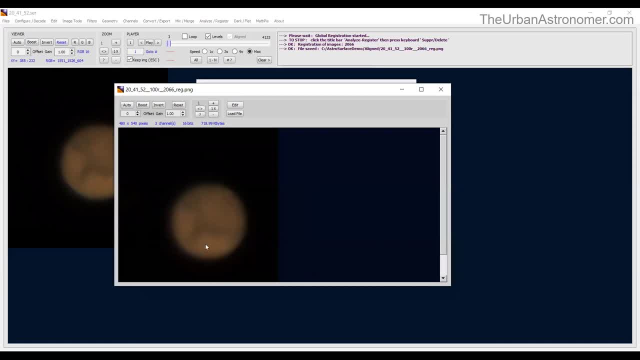 now, when we stack an image, even in order stacker, when once you look at the stacked image it is- uh, it looks a little bit blurry. so there are additional operations that we are supposed to perform. so in auto stacker, what we would do, we would take this file and then import it into. 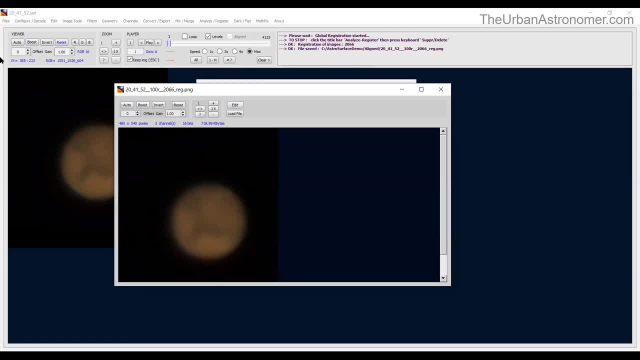 stacks and then do the waveform processing here. so the neat thing about um astrosurfaces that you can actually do the wave lip processing right within the same program. i'm going to click on edit of this file so it will ask whether do do i want to close the analysis options, which is that 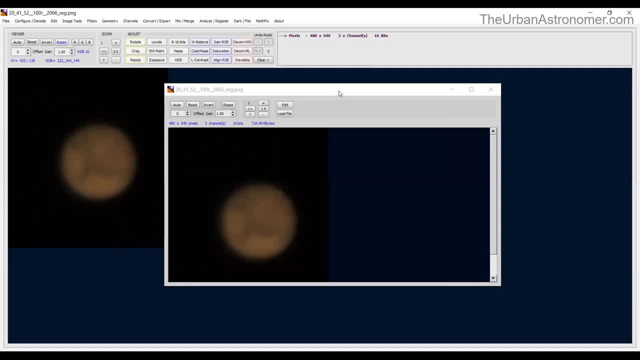 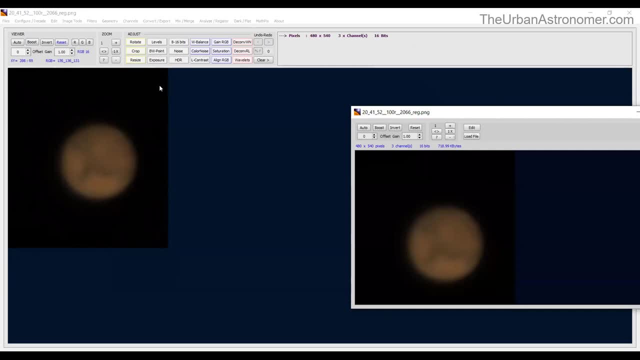 i will say yes. so now we are using the the. basically the stacked image has been opened in astrosurface. multiple options here that are now enabled and that we can use on the uh, on the image. so i'm just going to enable white balance initially, just a bit. 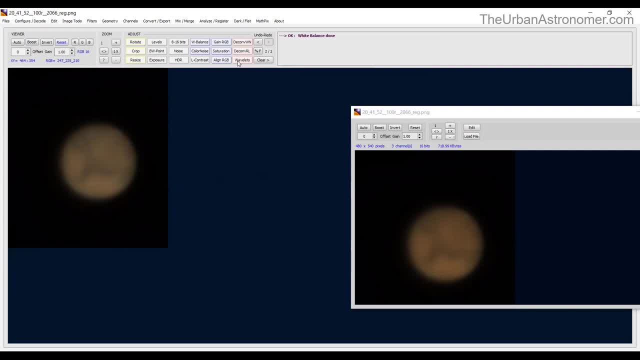 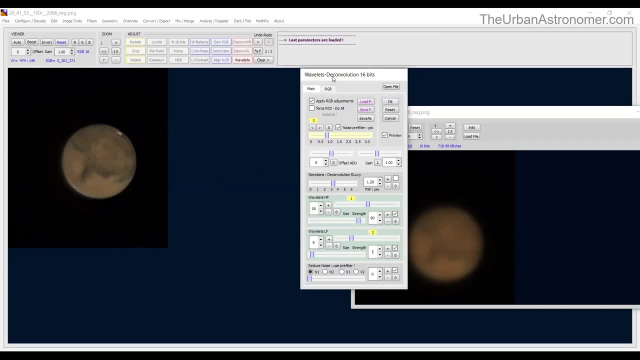 200 and say okay and i'm going to open the waivers. you can see that it has immediately transformed the image. the reason is that i was already playing with the wavelets and there is already some options applied, so let me just reset this and you can see it has gone back. 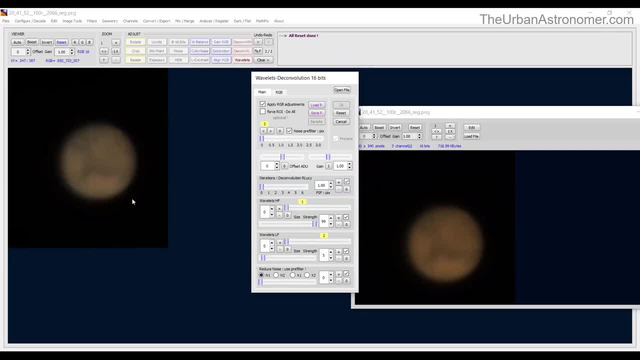 to what it was before. so there are multiple options over here, uh, to work on this image. so what i like to do is i will just enable wavelets hf. okay, i'm going to increase it and you can see that all the details are coming up nicely on the martian image. um, but you can see. 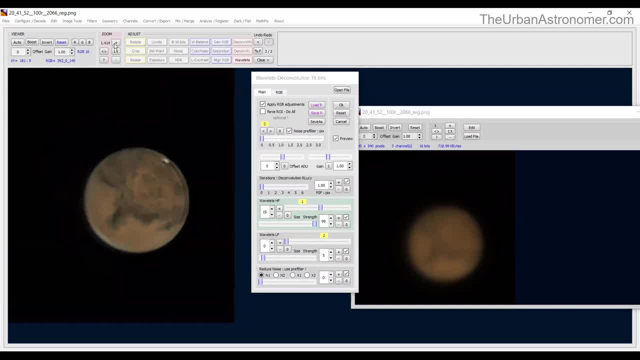 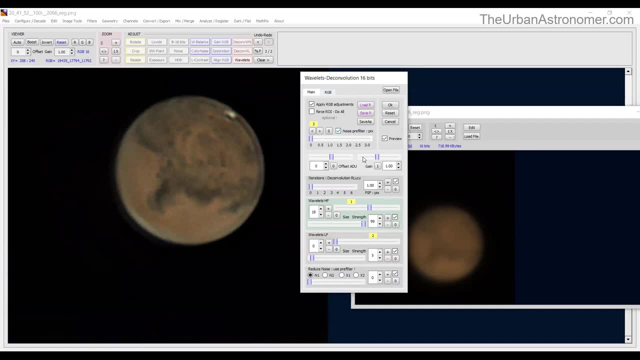 that it is a little bit noisy, so we have the option of zooming in, if you want, like this, so that we can take a good look at the image that we are working on. uh, so i'm just going to start using the noise pre-filter so that you can see that really. 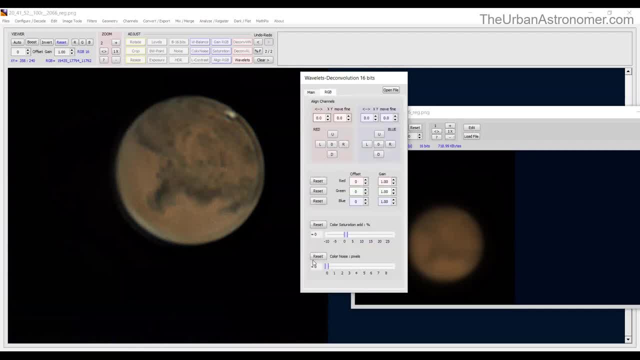 brings down the noise. in the image in the rgb section there is also color noise reduction, so you can use that if you want to further reduce the noise. there is also a wavelets lf that i'm going to use to increase the sharpness of the details. okay, so you can see this h rind effect. so that is a problem. 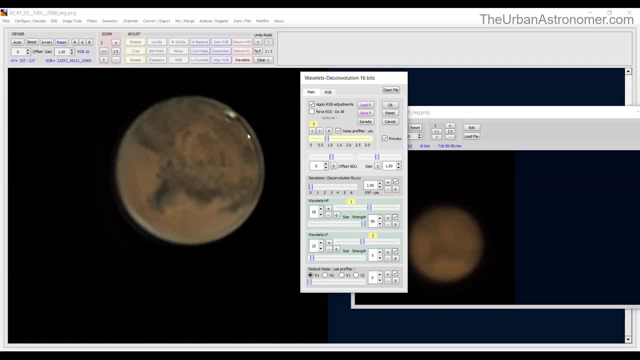 with pushing our telescope, so i'm just going to leave it as it is. i'm i'm not too bothered with that, so i will leave it as it is. we have additional noise filters over here, okay, so we can, so apply it a bit to just smoothen the image a little bit. okay, so let's look at it at 1x again. 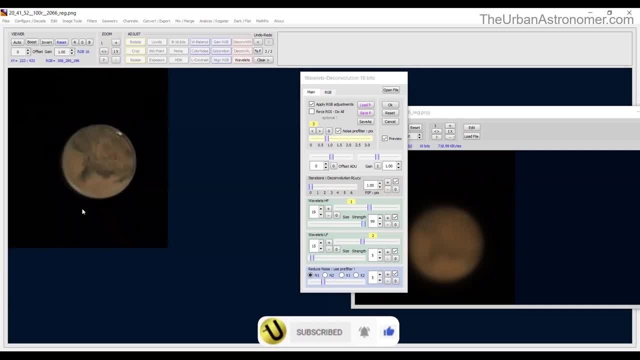 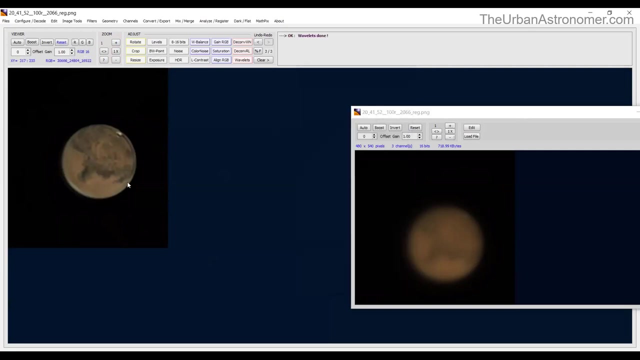 that is the martian image that i have right now, so you can obviously play around with these settings and then find what is the correct options for you. maybe i will just bring this down a notch to 92. okay, that looks good to me, so i'm going to say, okay. so now we have this image, which we can. 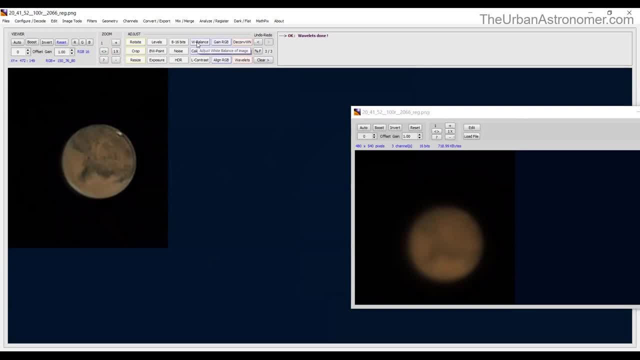 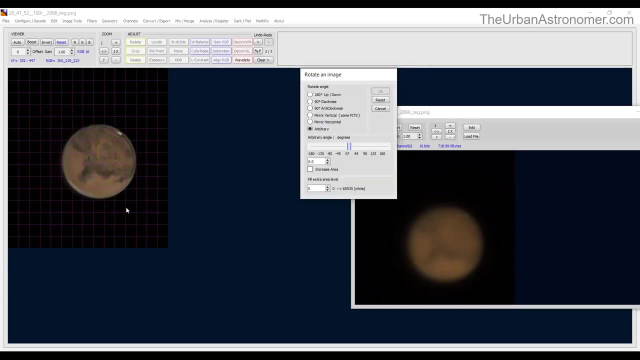 further work on. so now, if you want to do a white balance so you can see here that i took a white once more, you can see I'm just going to say cancel for now and there are other options, so I do want to rotate this. okay, so my image was basically flipped because I'm using a mirror in the image. 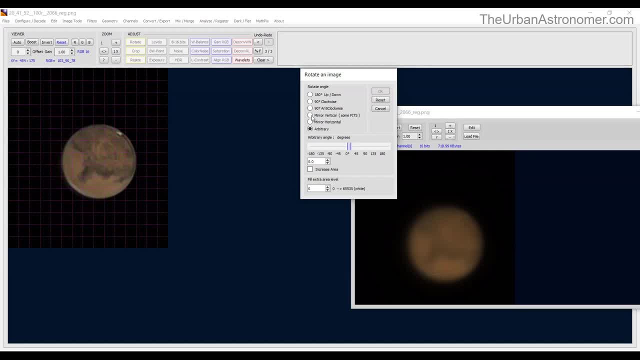 train in my diagonal. so I'm just going to, and that's not a good idea, but then I'm just lazy so I just use a diagonal in the train. so we have the option of something called mirror and it has flipped it okay and we have to click OK. 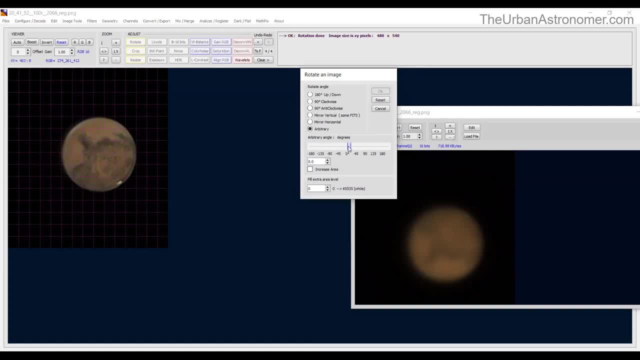 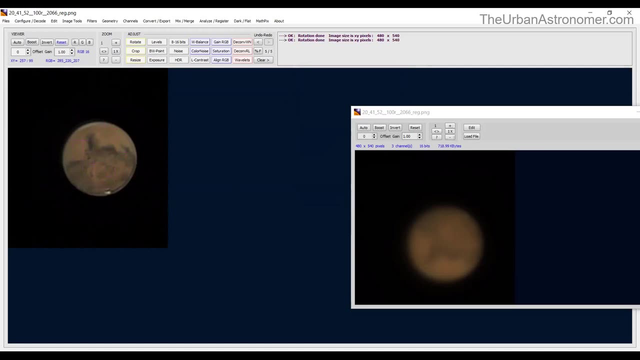 and if you want to rotate the angle, we'll have to rotate it again like this: okay, supposing I wanted to look like this, okay, so I'm happy with that and I'm going to say okay, okay, in the viewer we can basically click on auto and then it. 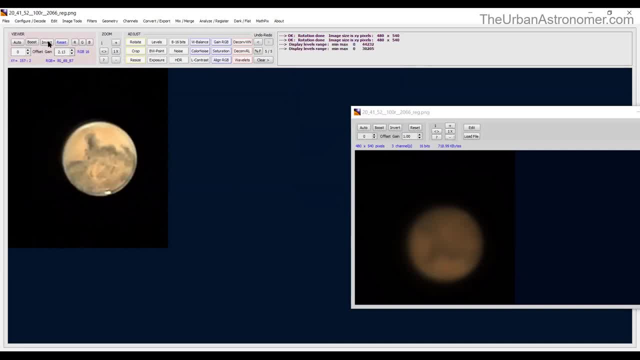 will auto-brand right and the image can also boost to make it even further, invert and then reset to original. then there are multiple options here, like we have resize, which is obvious what that does. and then there is and crop, there's the levels option which will automatically adjust the levels for you. so there is a 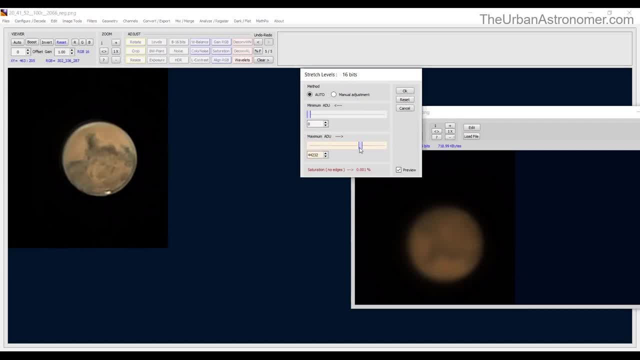 maximum ADU, minimum ADU and maximum ADU here that we can play around with to adjust it manually. okay, I'm just going to say auto and it has done that, so I'll just say okay. then there is a black and white point, ok, that you can select if you want. there is. 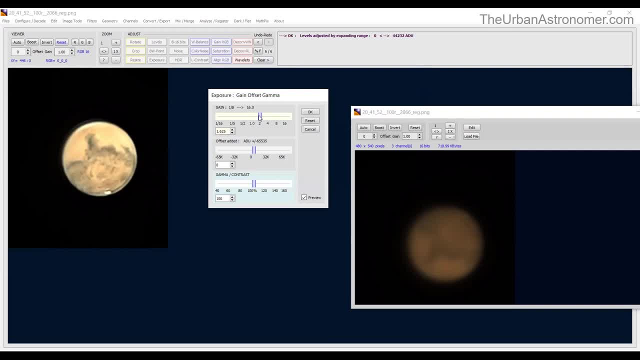 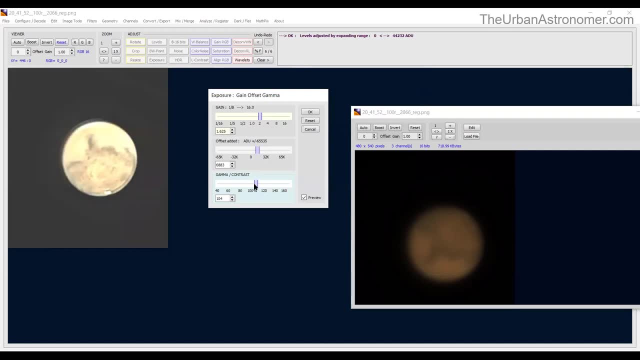 exposure. ok, so I can increase the gain or the offset or even the gamma contrast. so this will help bring out, for example, if there are moons- though in my footage I have not been actually able to capture the Martian moons- but in case of Jupiter, Saturn, things like that, these actually 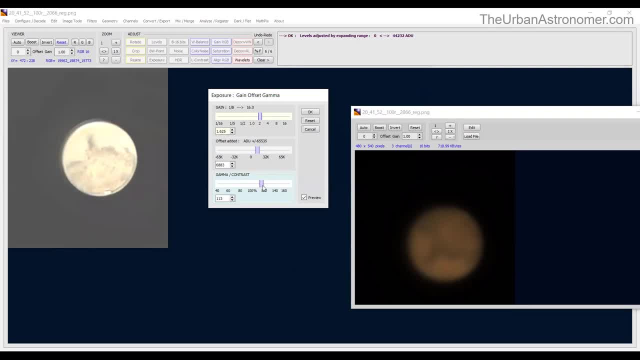 bring. help bring out. if you want to make a composite with the moons and the plant, these options can help bring out. yeah, you know the layer that you want to use for the moons, for example, you can. you can increase the contrast and look for it. okay, we're just going to reset this. then there are multiple noise. 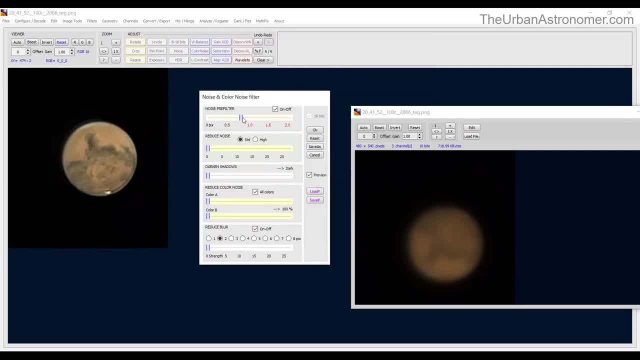 options over here. so there's a noise pre-filter. you can see it has become a little blurry and then you can apply the noise reduction. on top of that there is a dark and shadows option. you can look at the darker areas, what is happening and to the edge of the Mars. so these options are available. you can reduce. 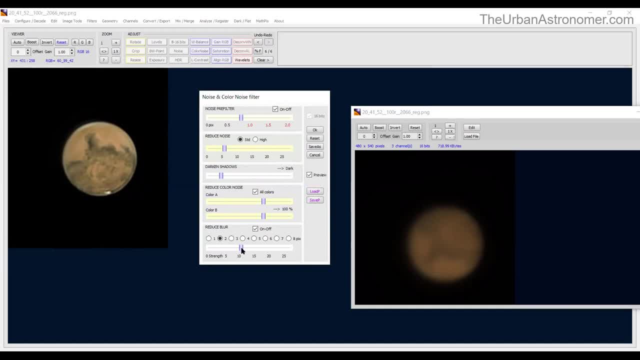 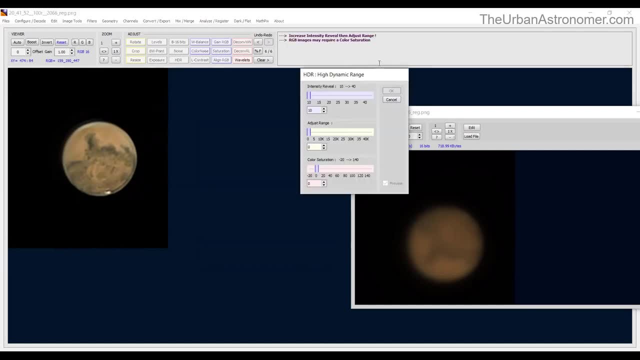 color noise over here and there is also a reduced blur option. you can reduce color noise over here and there is also a reduced blur option here, once you have. I'm not going to use these options for now, so I'm just going to reset it and cancel. there's a HDR option, so here we can do a bit of color. 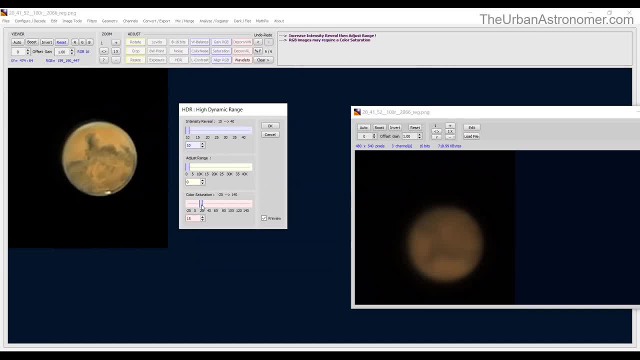 saturation. that, if you want, okay. so if I increase it to 15%, you can see the color saturation has increased. I like to use this on Jupiter and Saturn sometimes because it really makes the layers pop, because it really makes the layers pop okay, especially uses, okay. so I'll just apply white balance again and you can see. 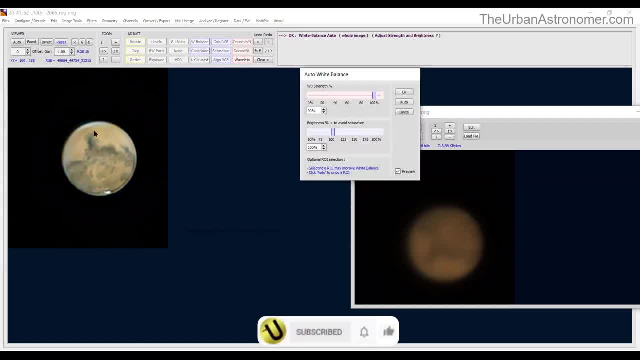 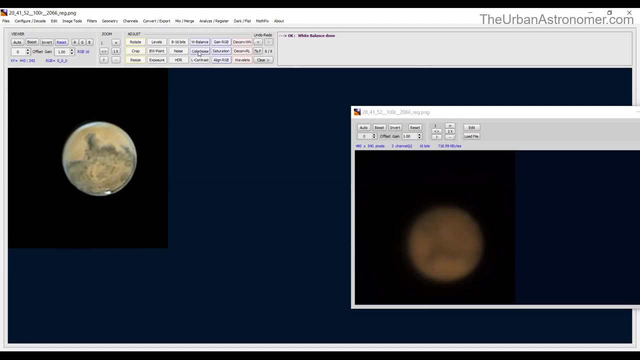 actually uses, okay. so I'll just apply white balance again and you can see these are actually clouds, so the clouds are actually turned into white now. so let's keep that. let's keep that, okay. then again, there are multiple options like color, noise, if you want to. 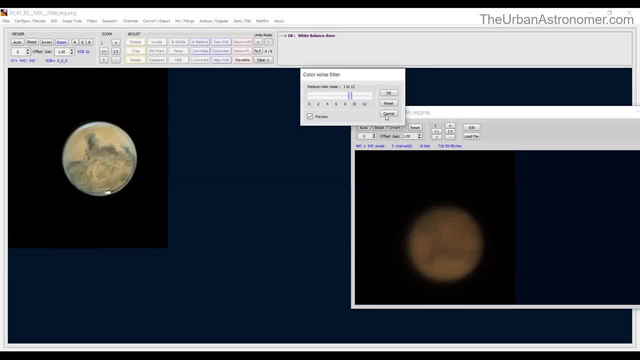 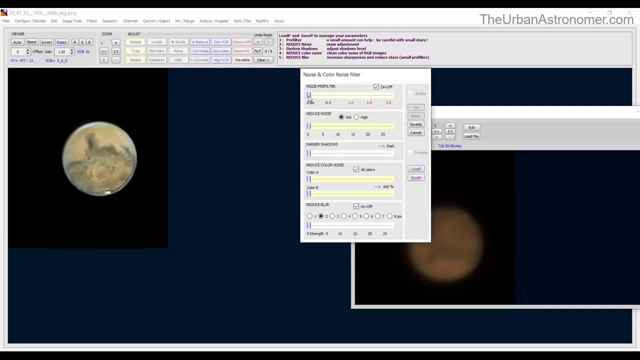 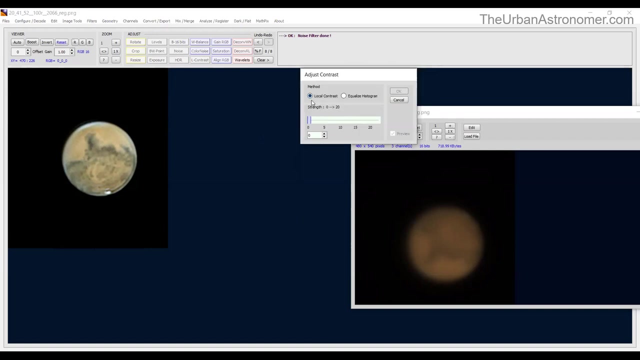 reduce the color noise in the image. okay, let me cancel that. it's become a little bit more noisy because of the saturation. let me go back to noise and just slightly decrease the noise in that, okay. okay, then there are other options, like a L contrast. okay, so we, here we. if you modify this, you can see the effect on. 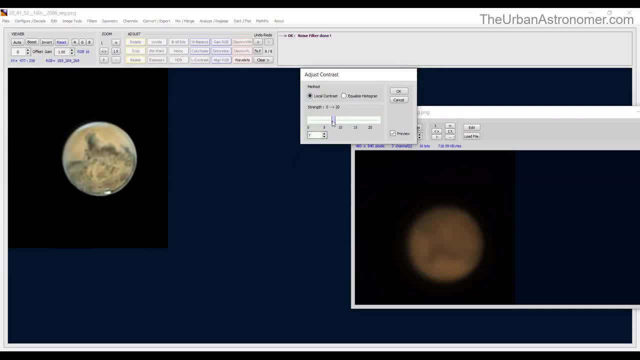 the image, so it is bringing out more details here, so it's something that, if you are interested, you can try it out. and there's also equalize histogram that is having different impact on the surface features over here. okay, so let me actually use a equalize histogram and 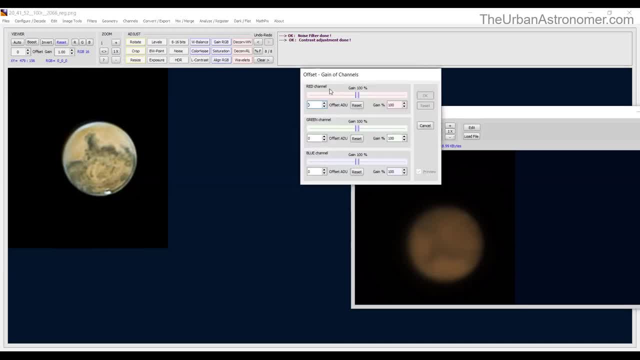 then there's a gain RGB saying: gain RGB. if you want to, you know, work on each of the channels individually so you can do that. so if I bump up the red, you can see that the planet is looking more red, or you reduce green, which is what I need to do sometimes. 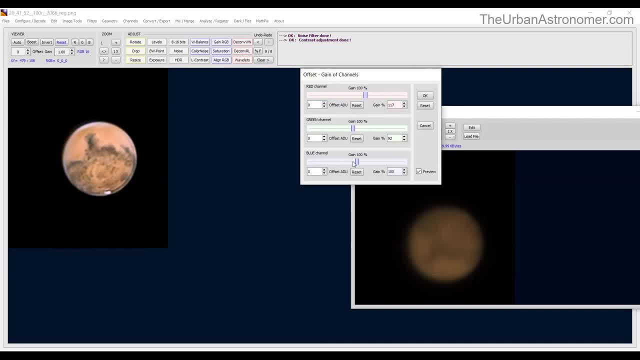 because the green is more sensitive on my camera- or increase blue decrease- I'm just going to reset it, cancel this saturation. this is again specifically working on saturation. you can increase the color noise pre-filter and then increase saturation and brightness of the image. and there's a lane RGB where you can select and then say a line. 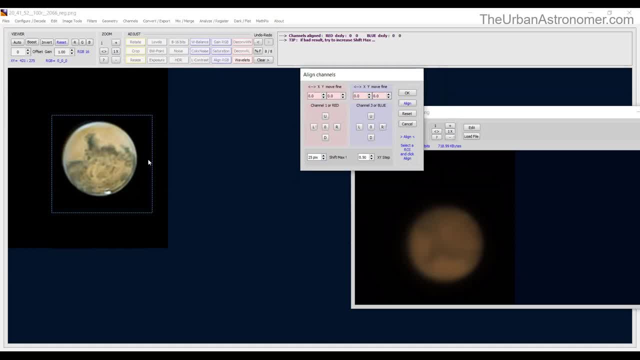 and it will do a line. so this is useful if you are working on Venus or in general. if your RGB channels are misaligned, then this will try and align it for you. then there are multiple deconvolution options over here which you can use if you want. 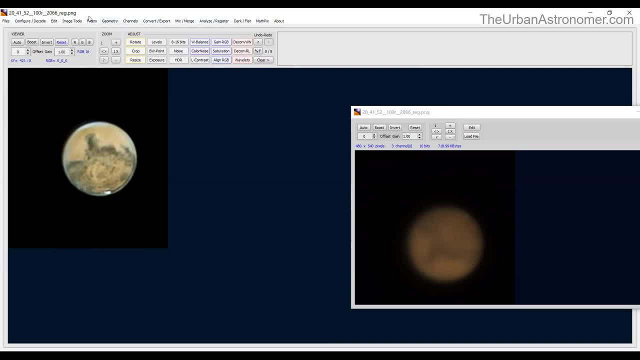 okay, I'm kind of happy with this image. so there are a lot of other options available. so like, for example, image tools, filters, geometry- some of them are common from here, others are not, so you can actually check for other options also. for example, there is something like perspective here, so this is interesting. 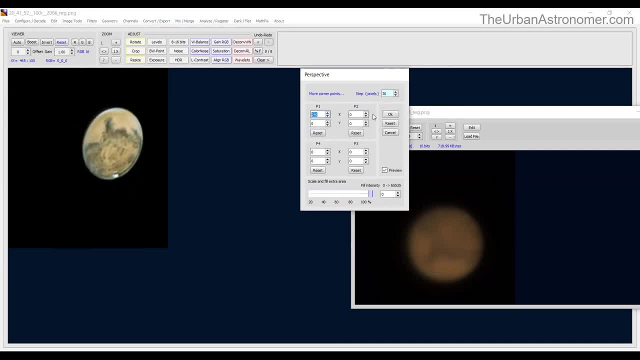 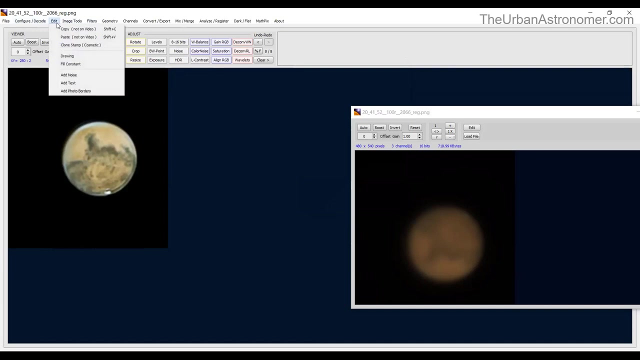 so you can look at what happens in case want, if you want your Mars image to look like it is flat, something of that sort, and we have a flat Mars, so these kind of options are also available. so there are some simple additional tools like add text. okay, so I 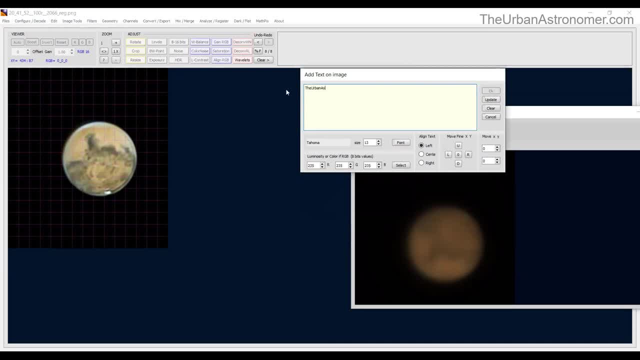 can just say: I've been astronomer. calm, you can select the font, do all that stuff. you can select the font, do all that stuff. you can select the font, do all that stuff. okay, so it is put it on the top. so if, wherever we want to place it on the 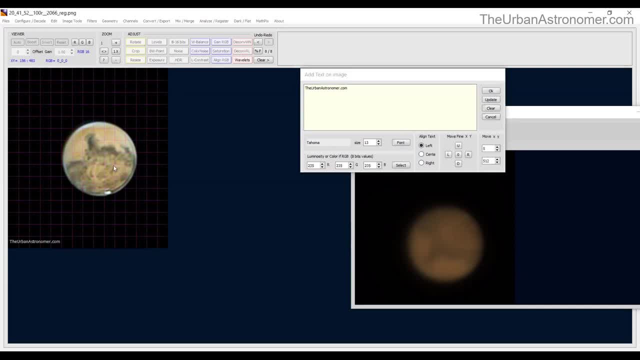 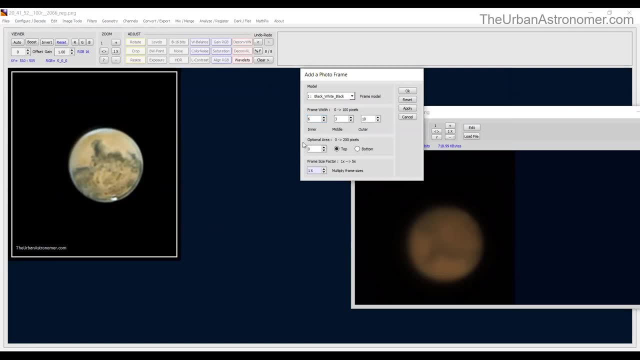 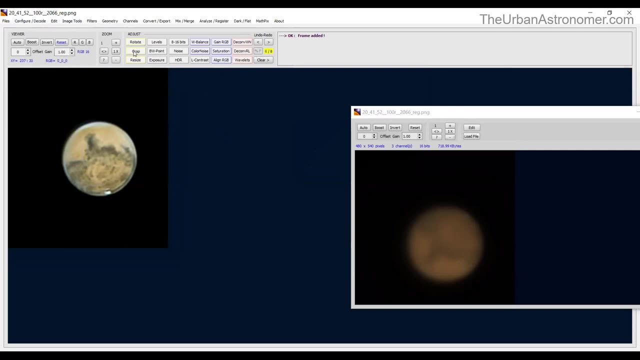 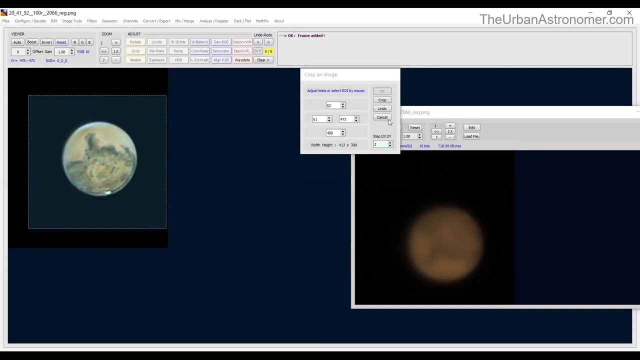 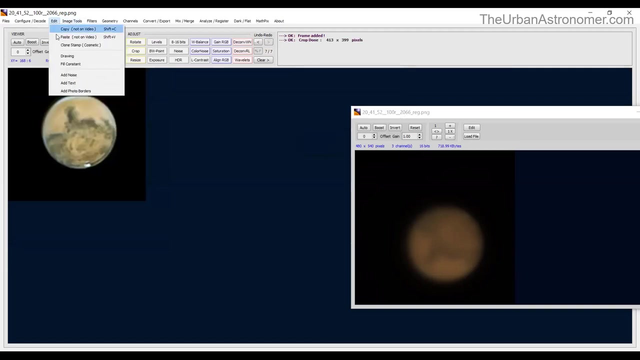 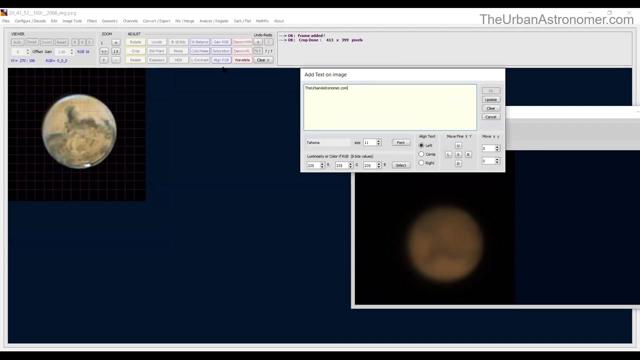 image. we just have to double click and it will place it on the image. there are also some options, like you know: adding photo borders, so like that. if you want to use that, see, let me undo that and crop this and I will click it. it will come over there. I will say okay, and if you want to, 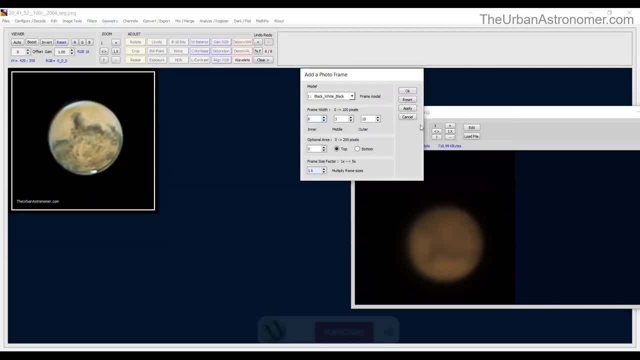 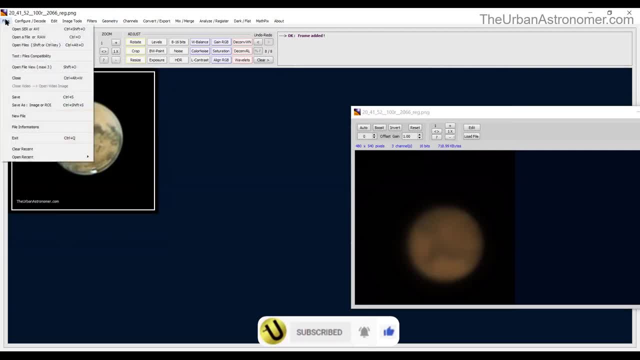 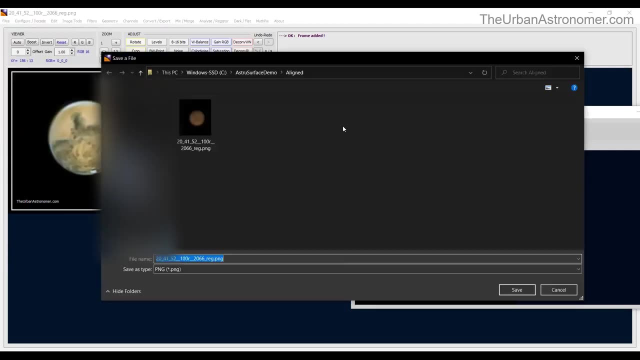 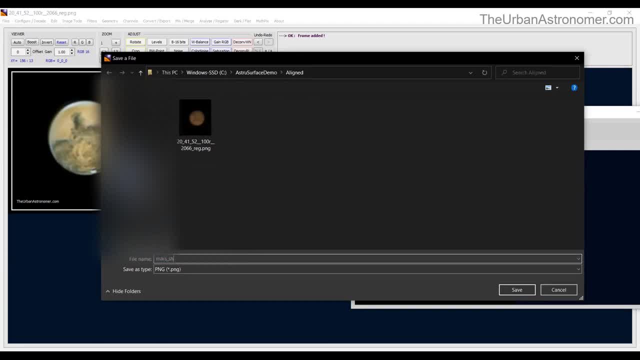 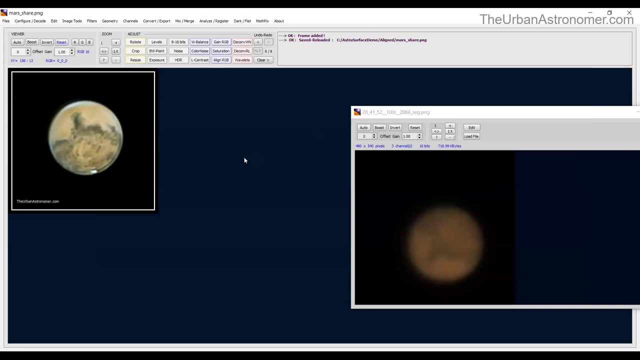